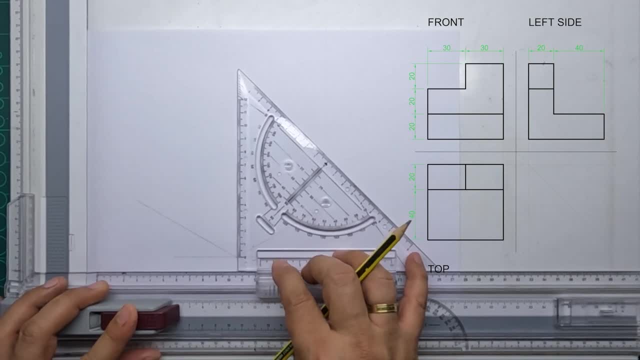 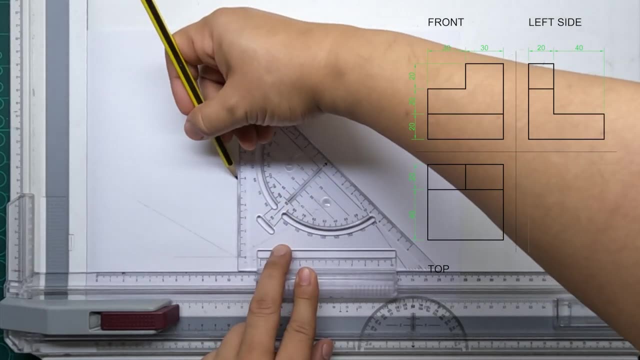 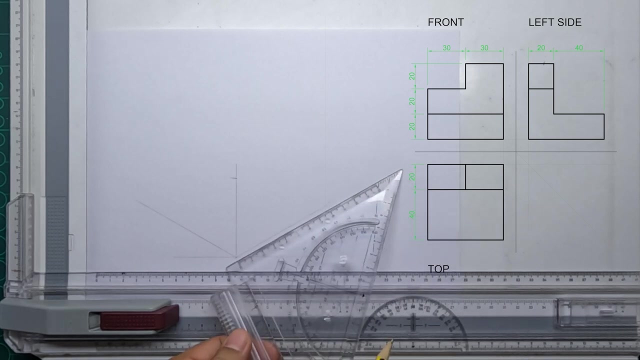 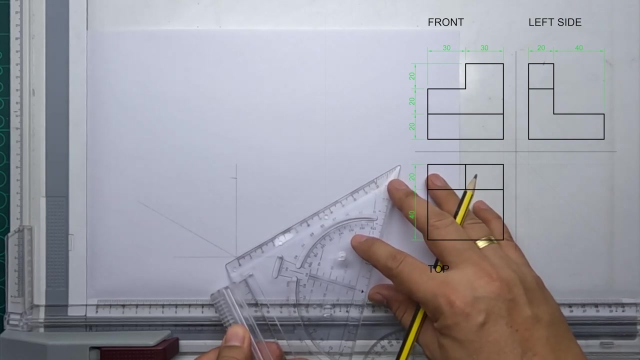 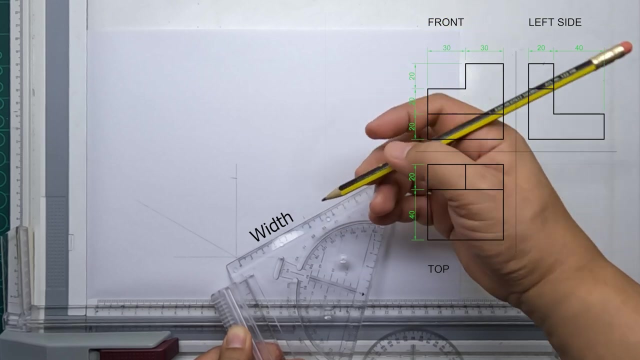 Next we will establish our three main dimensions of our isometric box. First we're gonna help the height. We can determine our total height from our front view in our orthographic drawing. Next will be our width. We can also get our total width from our front view. And. 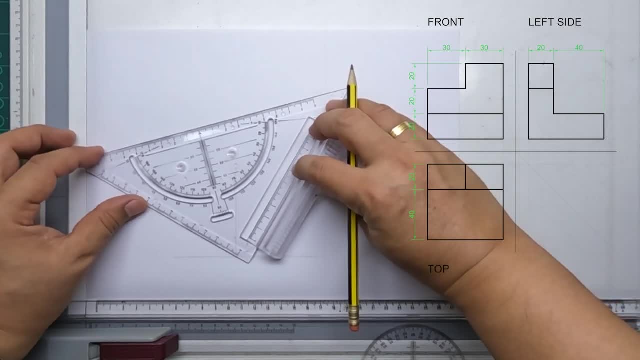 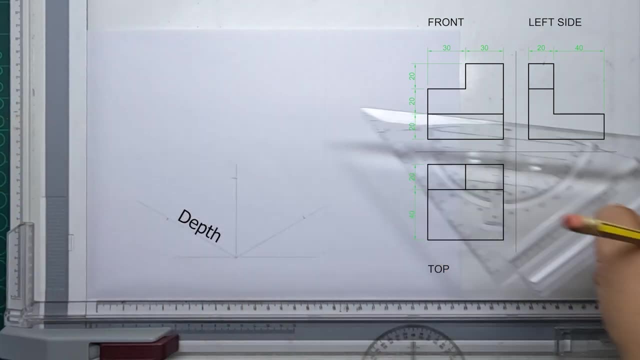 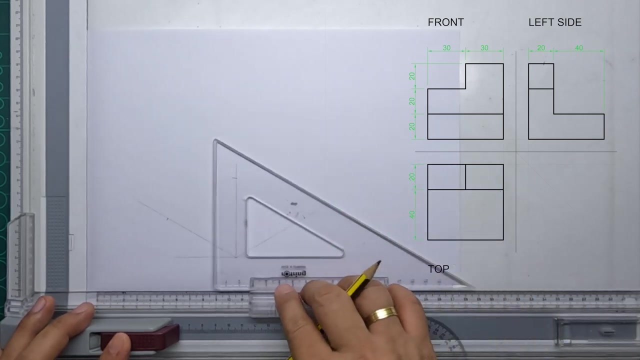 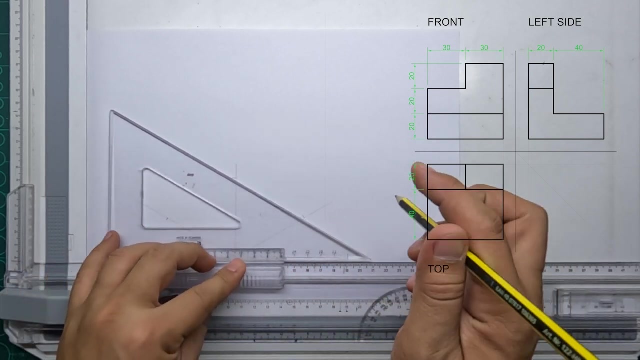 lastly, of course, our depth. You can determine the total depth from our top view. Next, we'll draw some thin lines in our drawing, On our left side of the Australians, on our right side of the Australians, And we make aват of 그렇지ing lines. Now, of course, we will get into to the 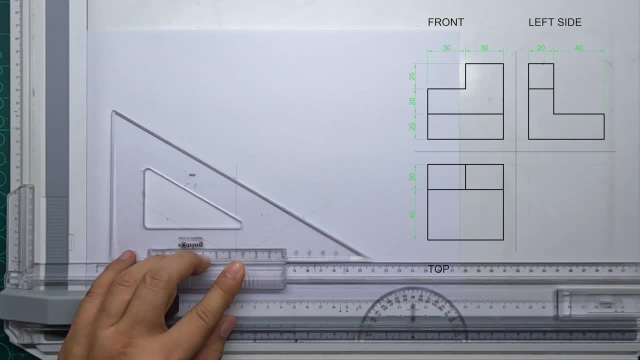 a little vehicle training, We can actually watch our videos by° representing our POC. A little car, a little light bath by us, And all that is done up to the point where our isometric line is locatedifting us to equation 3.. So we'll have pixels in there to rawn completion protein, and then we want auto-phyloque thwacks normalizing how a viewwick looks like. Now that we've established our 3 main dimensions, all we gotta do is to project all those points. with the help of our 30 by 60 degree triangles, We're gonna draw another inclined line going to the left. With the help of our 30x60 triangle, we're gonna draw another inclined line going to the left. 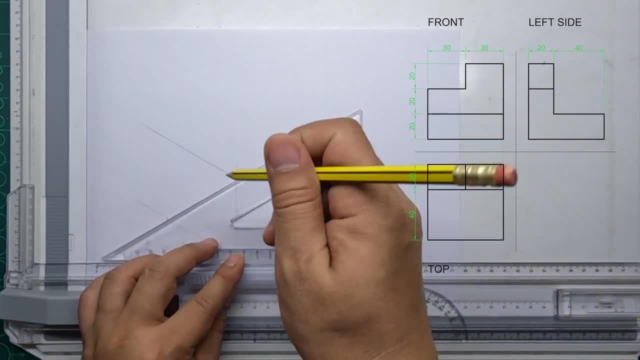 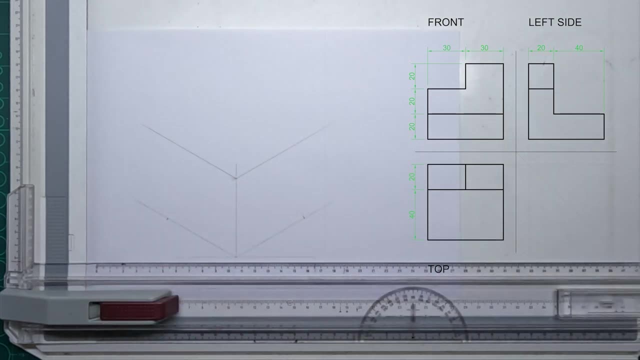 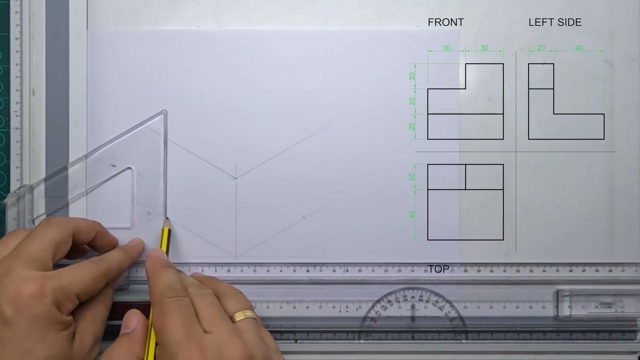 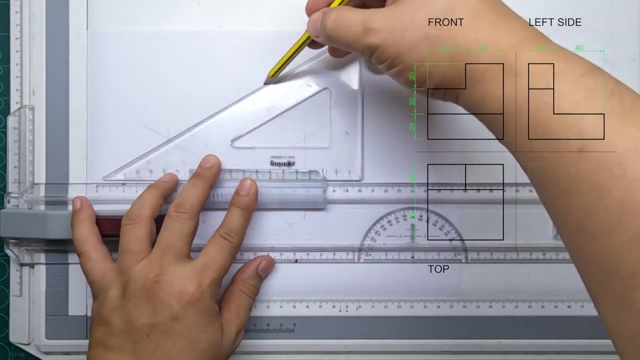 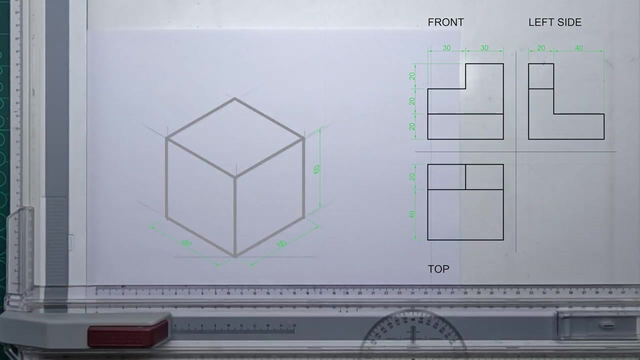 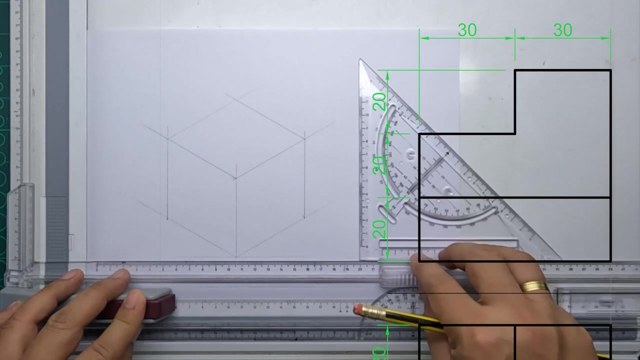 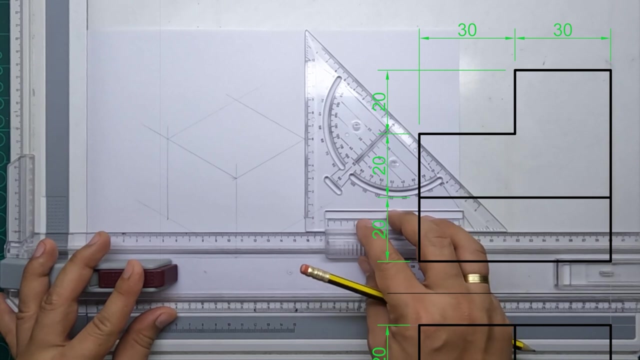 and another one going to the right. now we have our isometric box. now save, save. now save. example: our observer is standing right in this position. the red arrow indicates the front view. now we will take our measurements from our front view. we'll just follow all the measurements indicated in the front view. 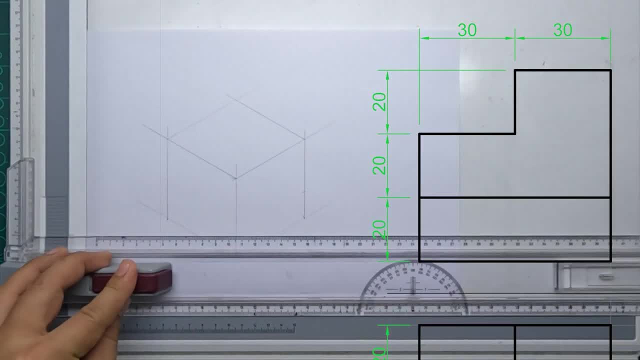 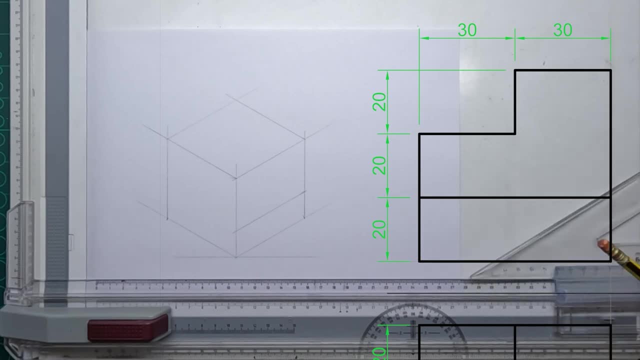 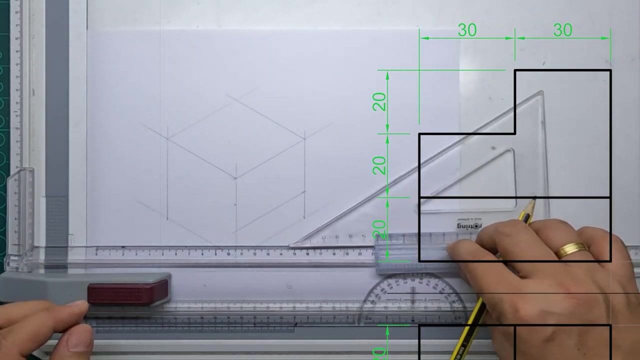 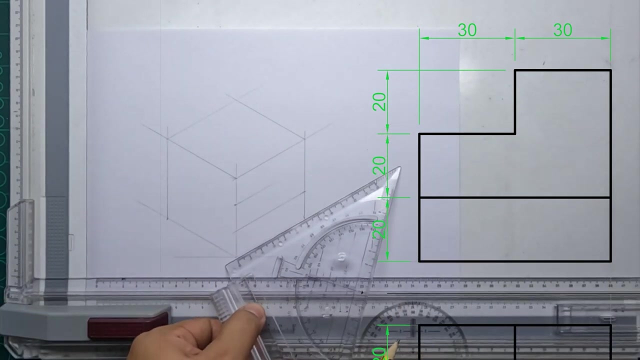 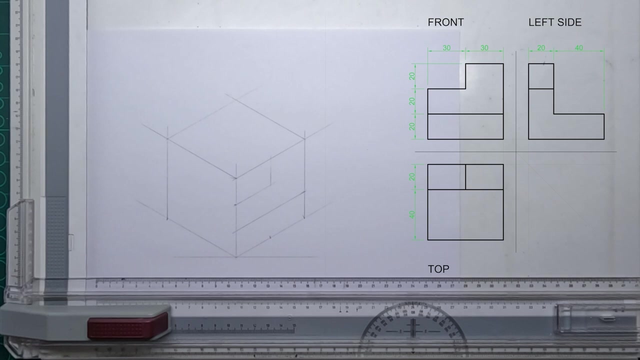 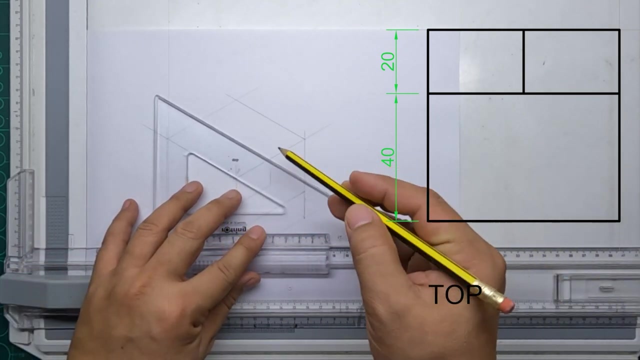 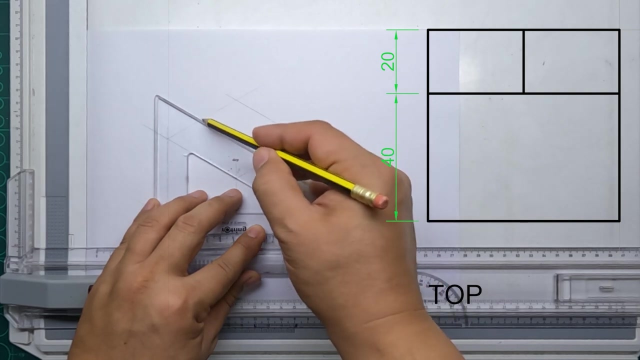 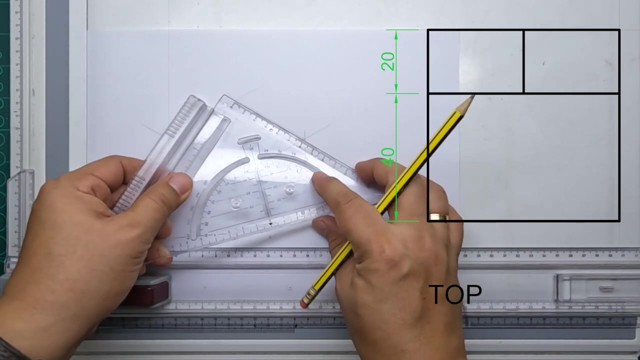 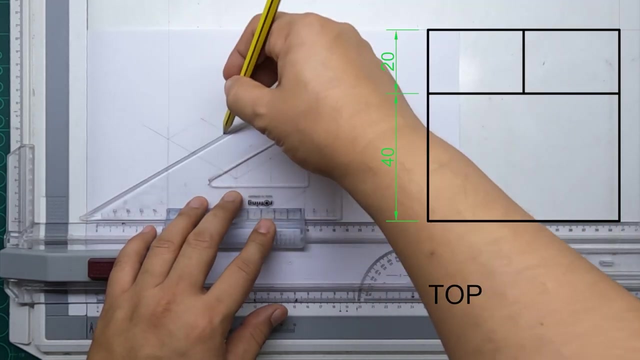 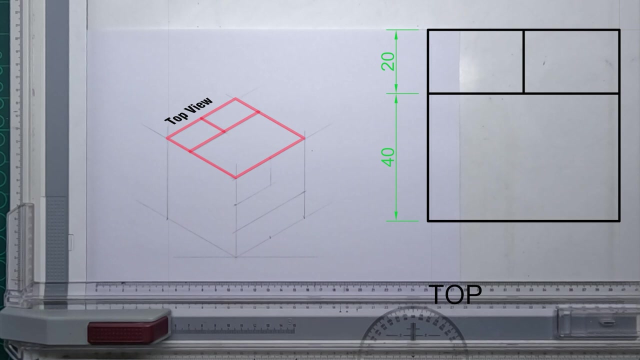 so so all right, we now have our front view. next to our front view, of course, our top view. top view is directly above our front view. again, all we need to do is to follow all the indicated measurements from our top view. there you go, we now have our top view. 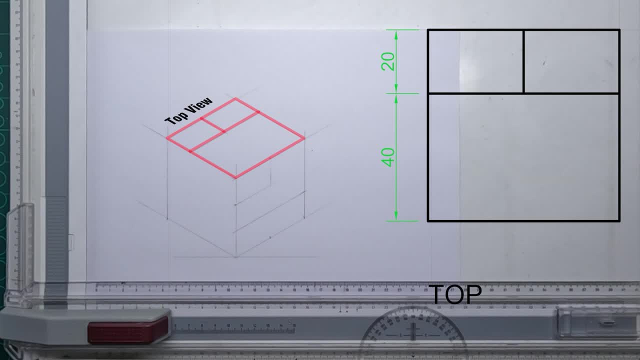 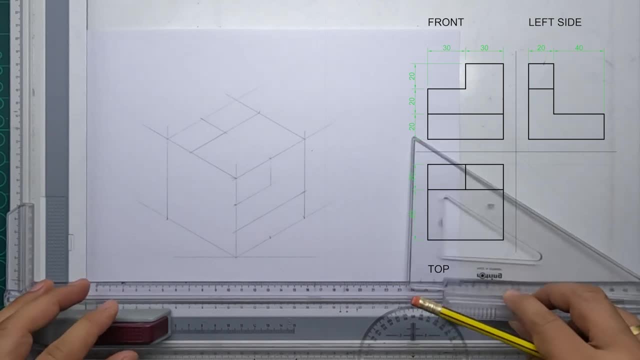 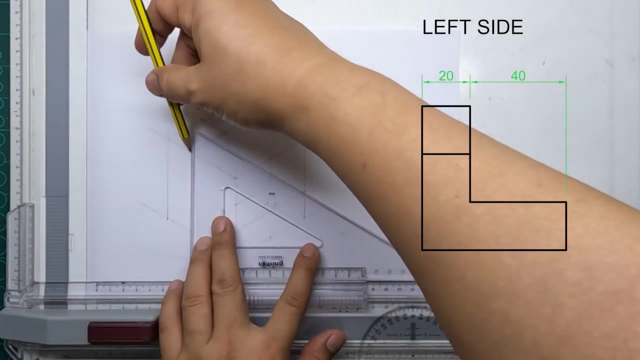 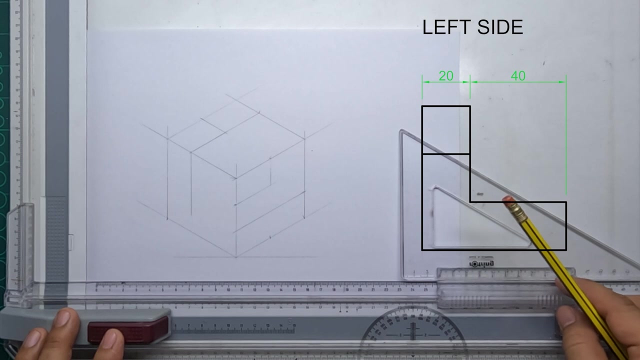 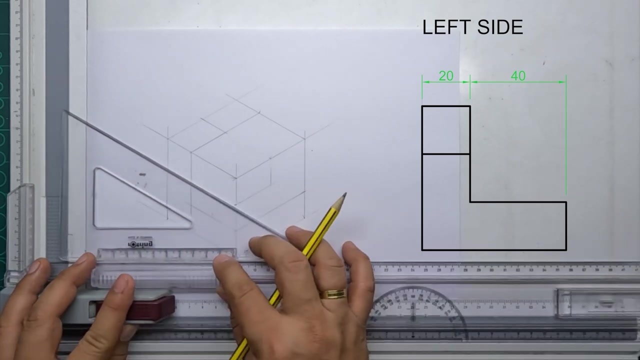 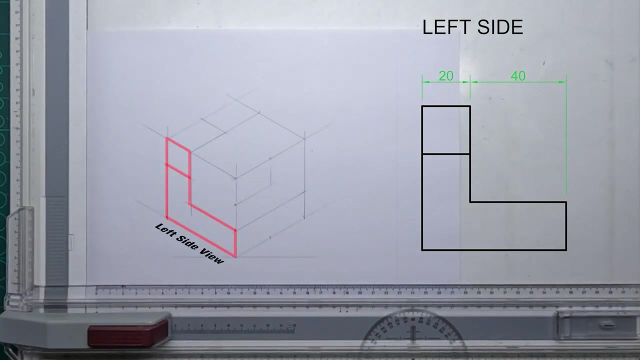 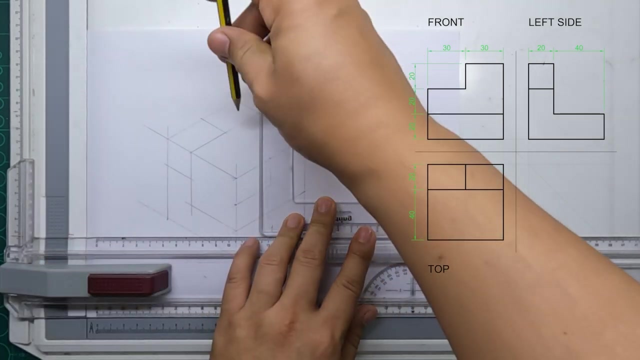 of course, next to our top view. lastly, we have the left side view. again, we will just follow the indicated measurements from our left side view. so, and there you have it, our left side view. now we completed all the three main views of our orthographic drawing, thrown in our isometric figure or isometric box. all we have to do now 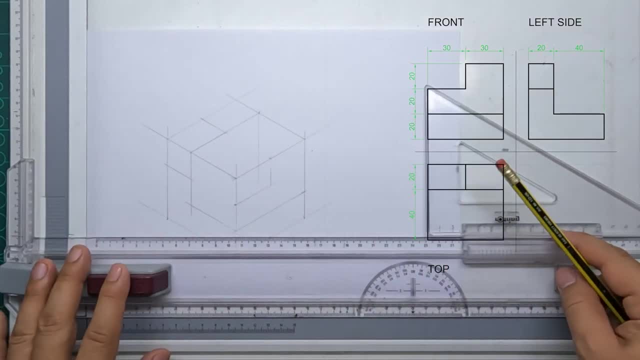 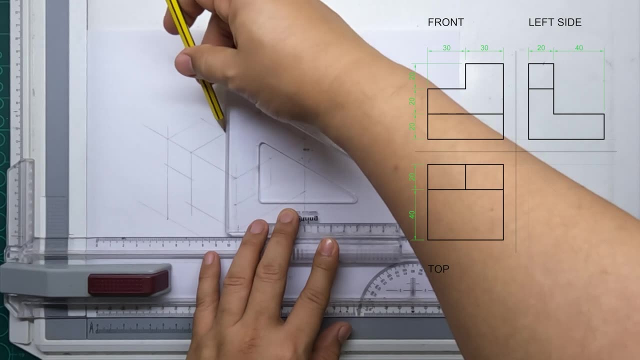 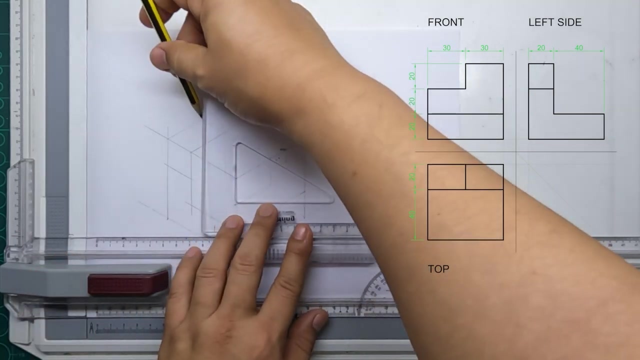 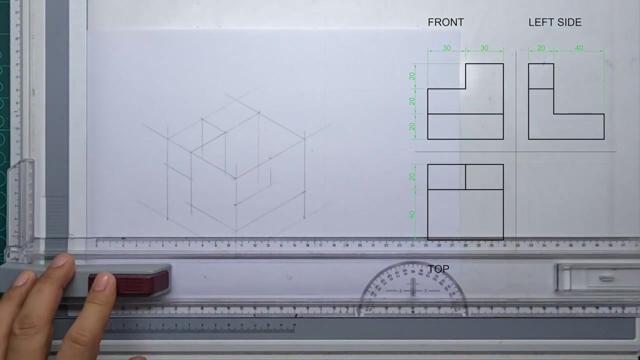 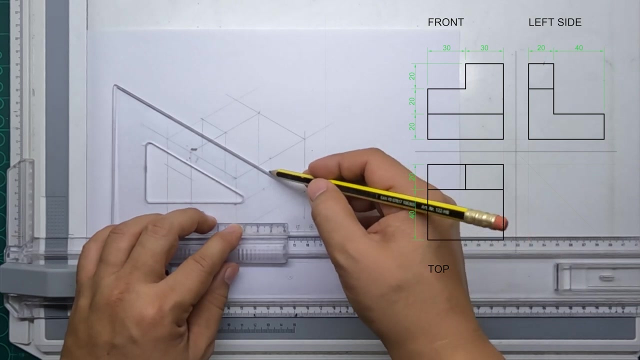 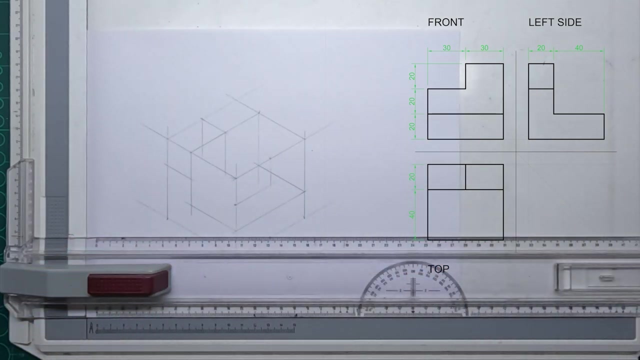 have to do now is to project all the contours and all the corners from those views with the help of our 30 by 60 degree triangle. first, I am drawing all the vertical lines from all the corners from our top view going down. the next, with the help of our 30 by 60 degree triangle, now, all the corners from 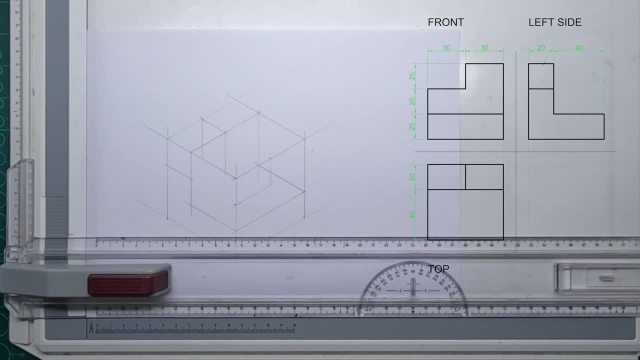 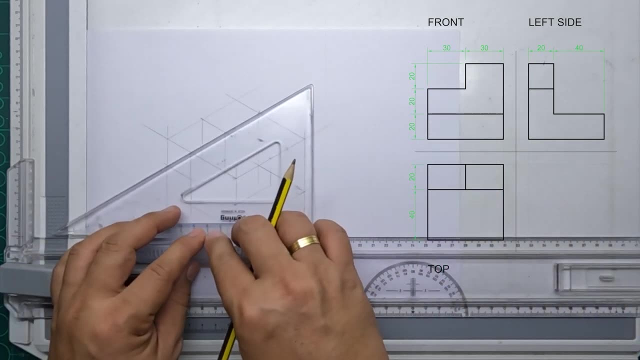 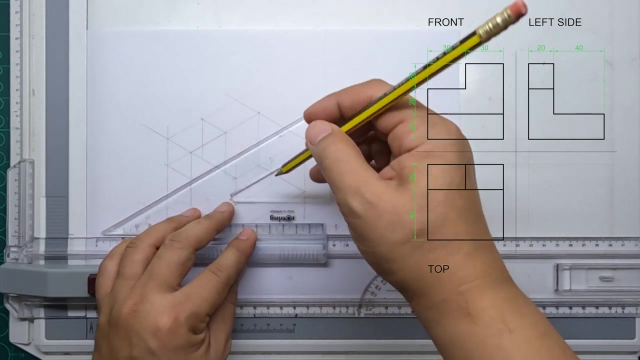 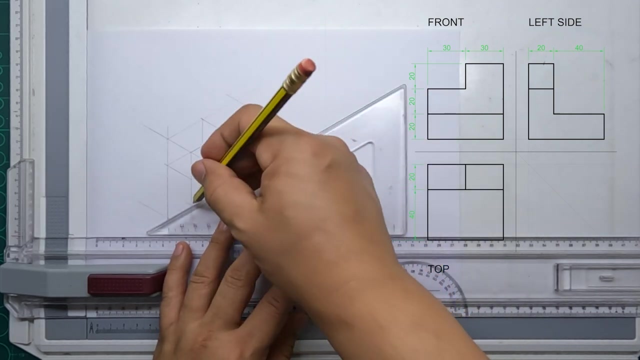 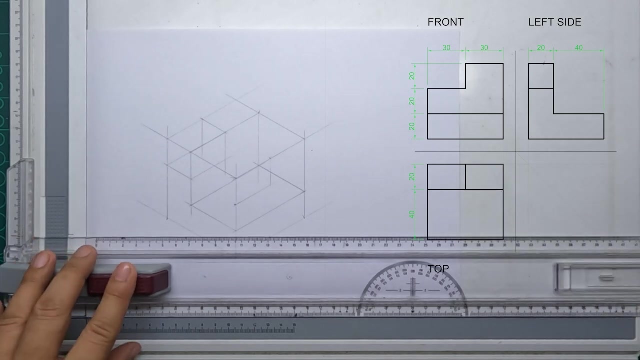 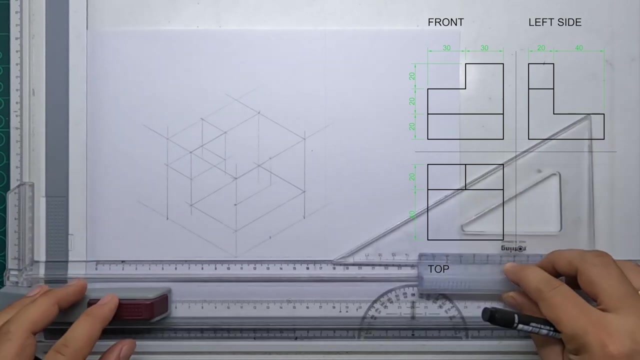 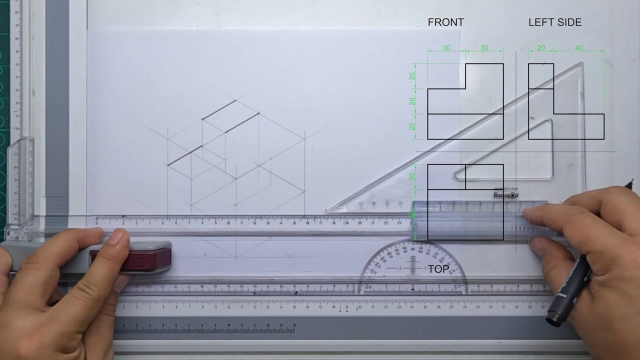 our front view. and now I will use my 30 degree by 60 degree triangle to project all the corners from our left side view. lastly, all you have to do now is to connect all the corners in our drawing. connect all the corners from corner to corner. 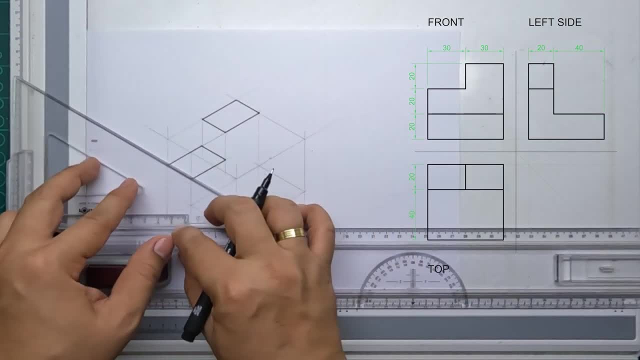 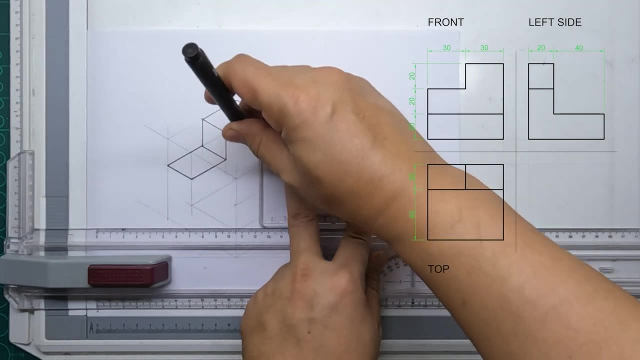 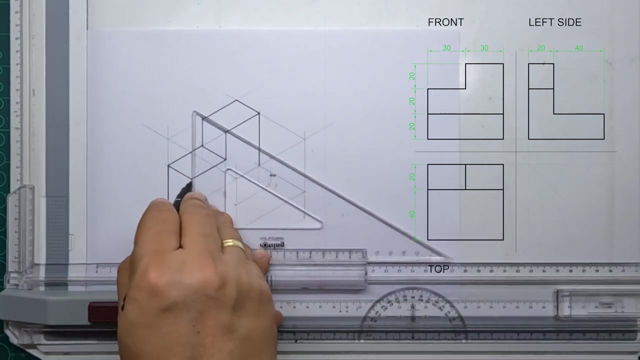 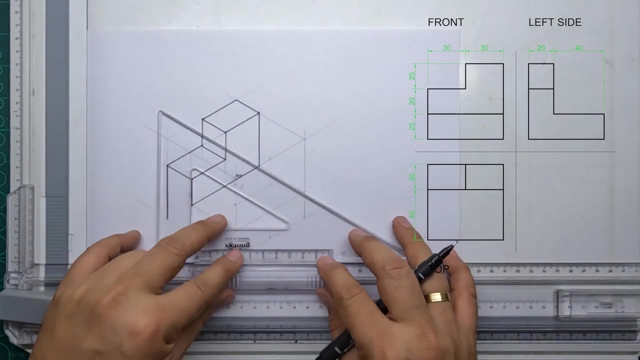 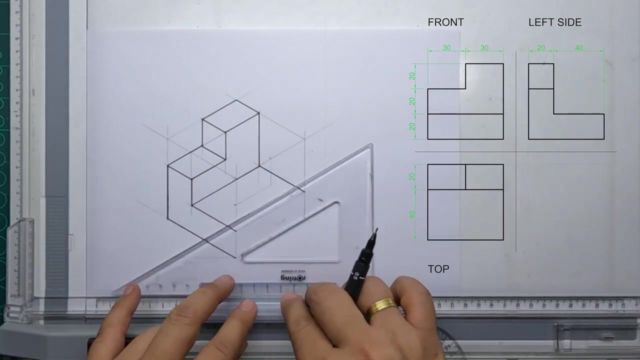 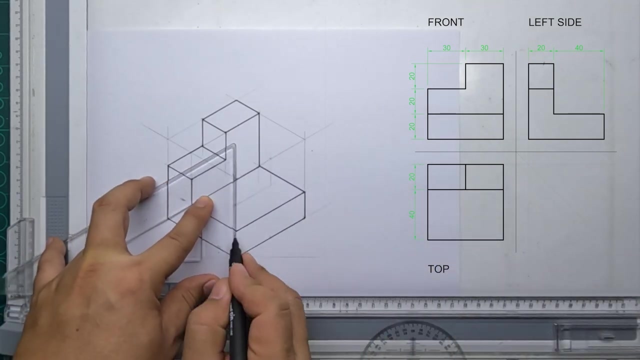 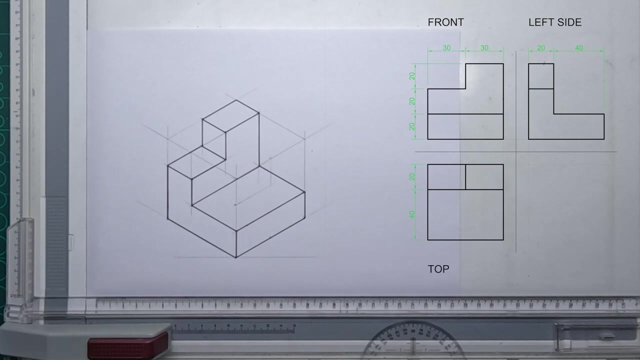 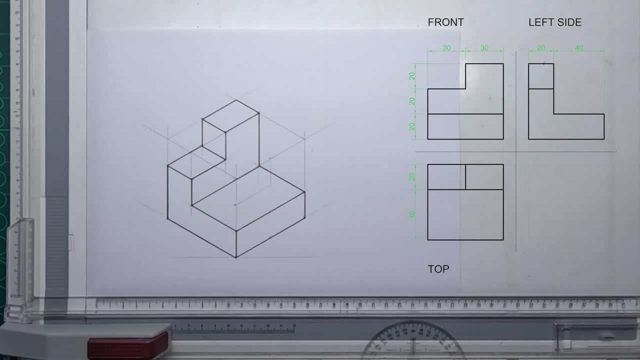 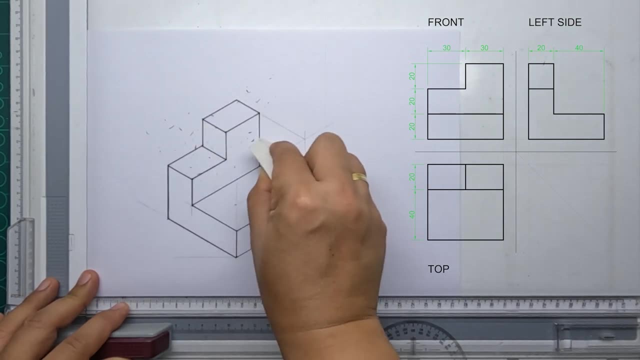 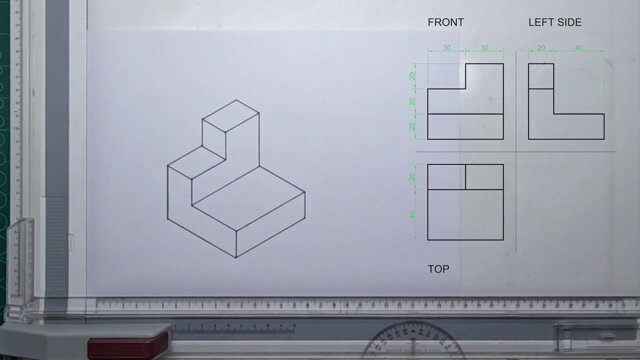 drawing and of course, you can always clean it up and you can always erase the unnecessary performance of a computer pencil lines. I hope you guys learned and enjoyed our video for today. For more videos like this, don't forget to hit that like button. share with your friends. 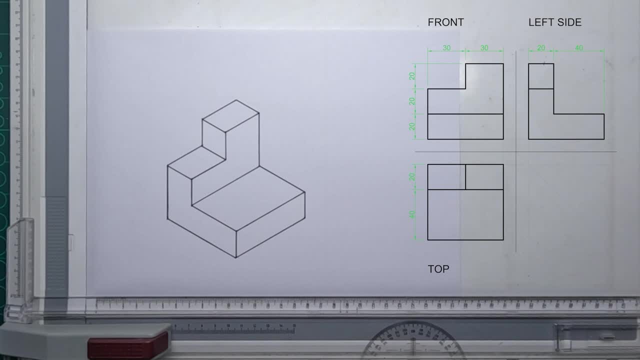 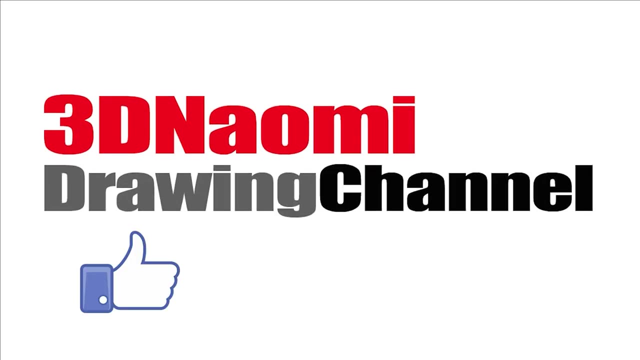 and, of course, subscribe. Thank you, Thanks for watching.